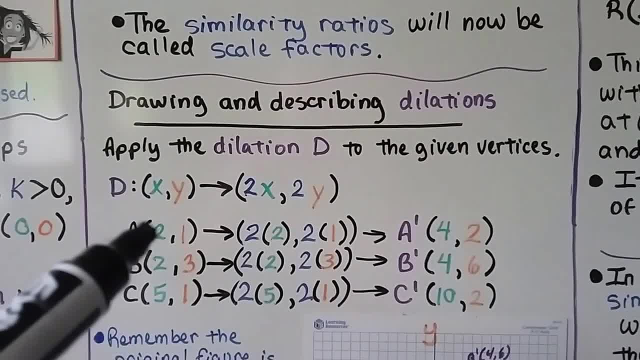 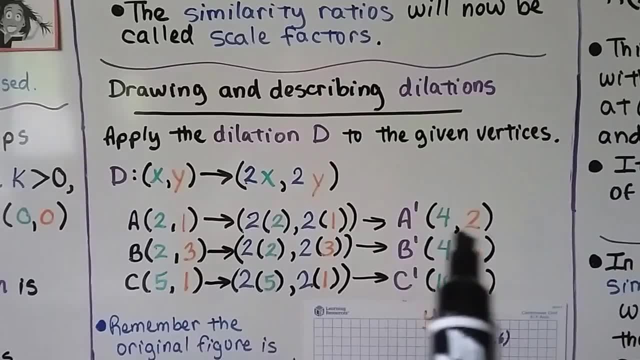 So we have a, b, c. a is 2 for x and 1 for y. We're going to multiply the x times 2 and the y times 2 for each one of these, And a prime is going to be 4, 2.. 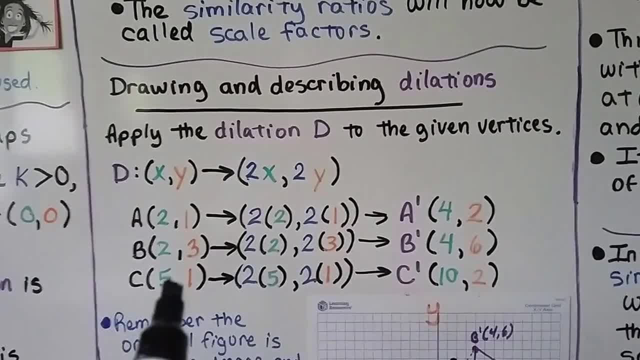 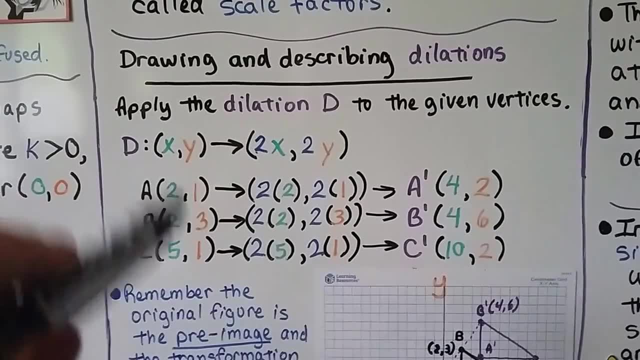 b is going to turn into b prime, that is 4, 6.. And c, that is a 5, 1,, is going to be c prime, that's a 10, 2.. And we can graph these points, and we can graph these points. 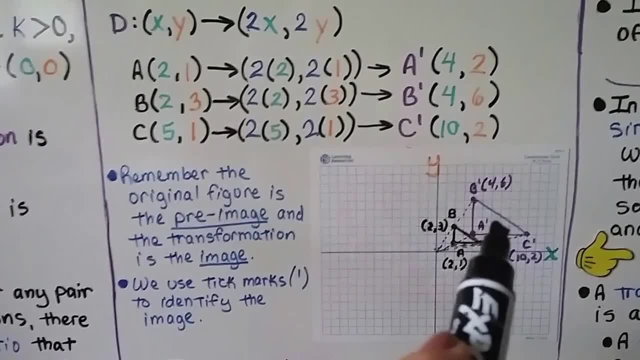 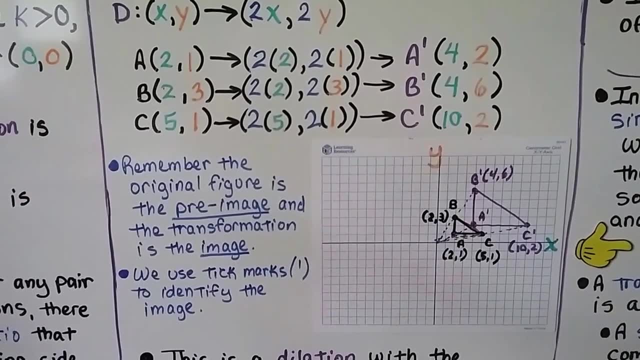 and we get this black triangle with a prime, b, prime, c, prime as this purple one. okay, So remember, the original figure is the preimage and the transformation is the image. that's the copy, And we use tick marks to identify the copy, the image. okay. 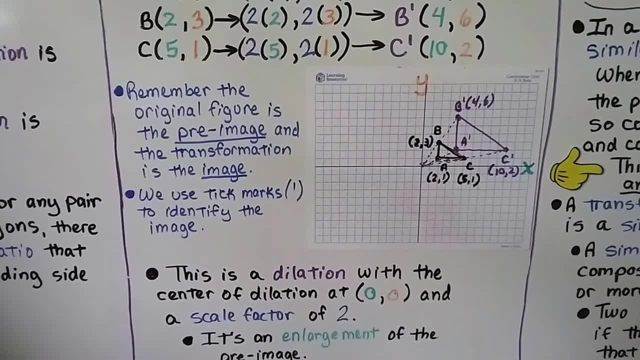 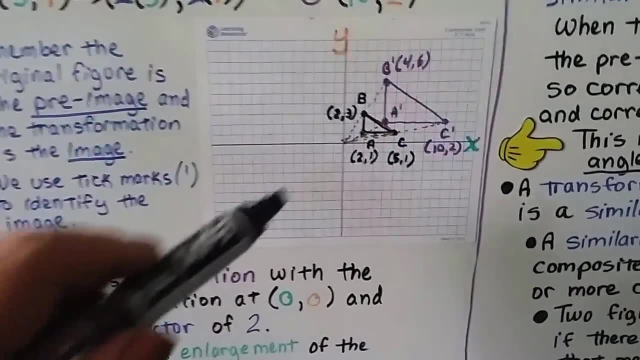 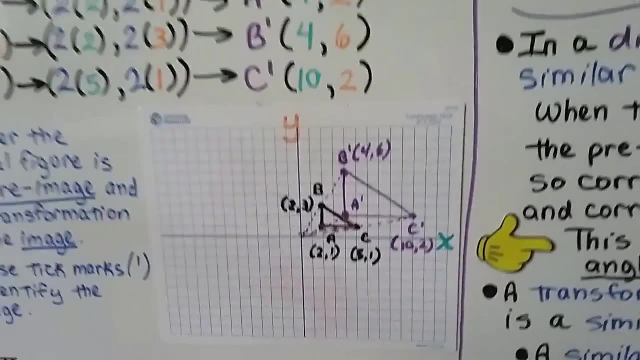 So this is a dilation with a center of dilation at 0,, 0, that origin and a scale factor of 2.. Okay, It's an enlargement of the preimage. So the preimage, the black one, enlarged times 2 and became a prime, b prime, c prime. alright, 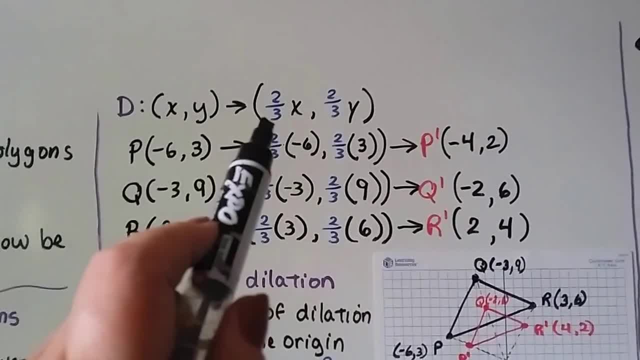 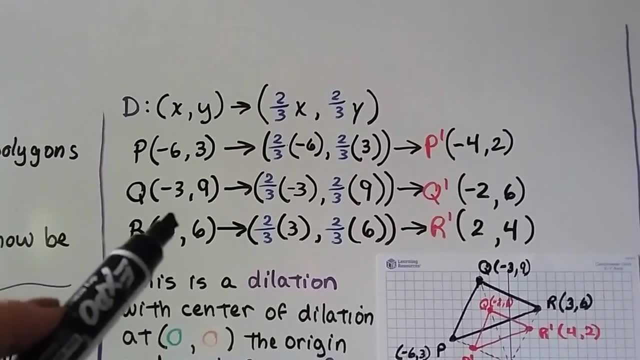 Here we have a dilation d, but we're supposed to multiply our x and y values by 2 thirds. Ooh, that's less than 1.. So we have p, q, r and the ordered pairs. When we multiply each of them by 2 thirds, we get p prime, q prime, r, prime. 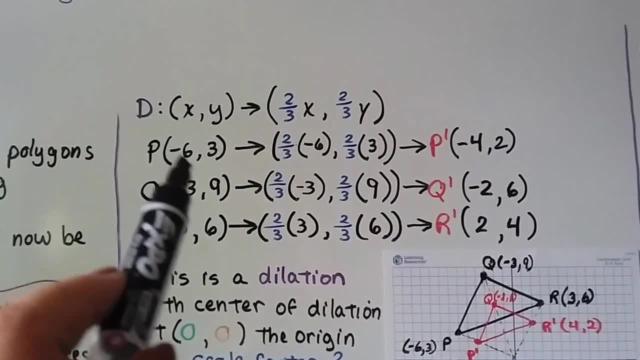 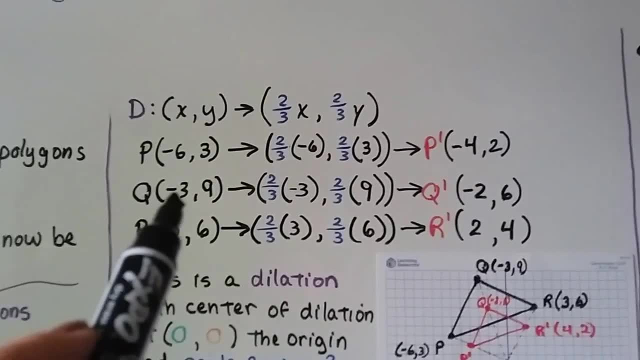 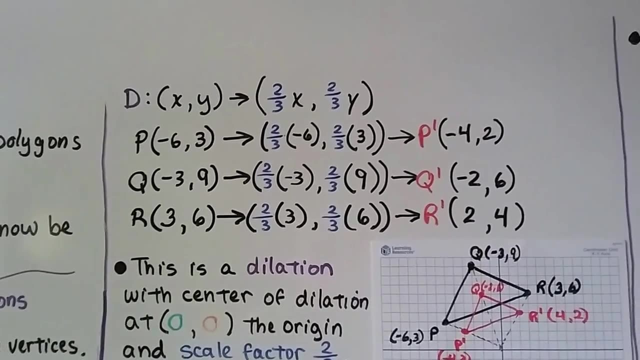 And look p, q, r. p went from a negative 6 for x and a 3 for y to a negative 4 for x and a 2 for y- That's smaller, alright. And q went from negative 3, 9 to negative 2, 6, and r went from 3, 6 to r prime as a 2, 4.. 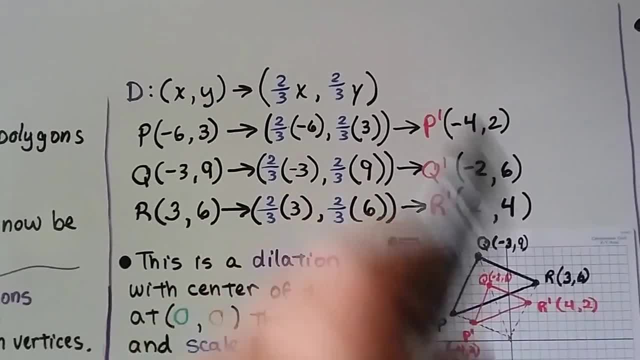 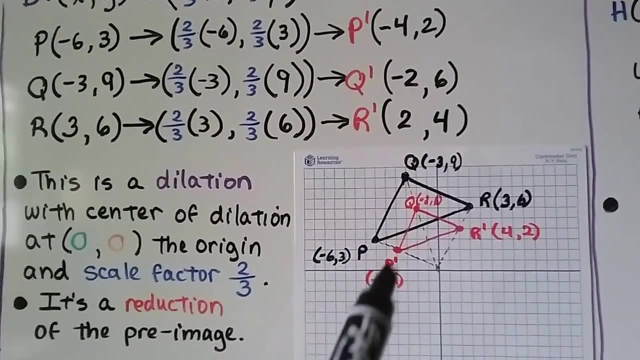 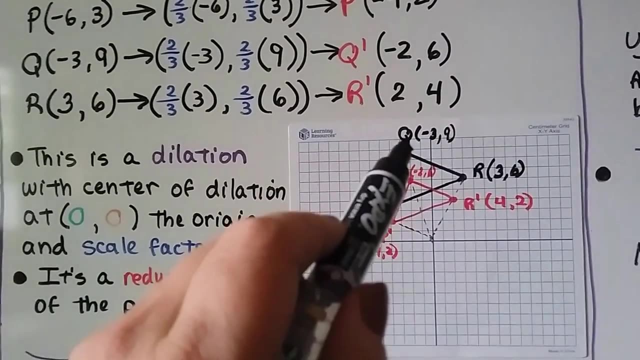 And we can graph these ordered pairs and these ordered pairs. So p q- r is the black one and p prime, q prime, r prime is the littler red one. When we draw lines from the origin through p- prime to p and through q- prime to q and from r- prime to r. 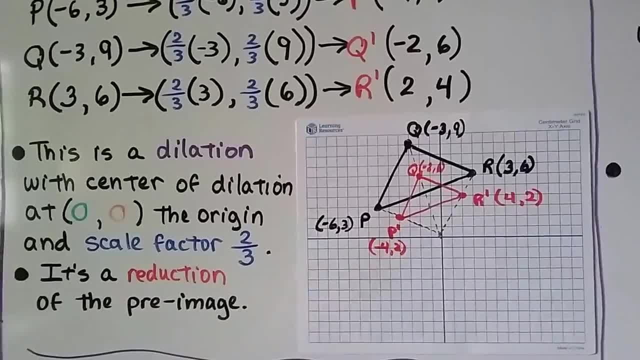 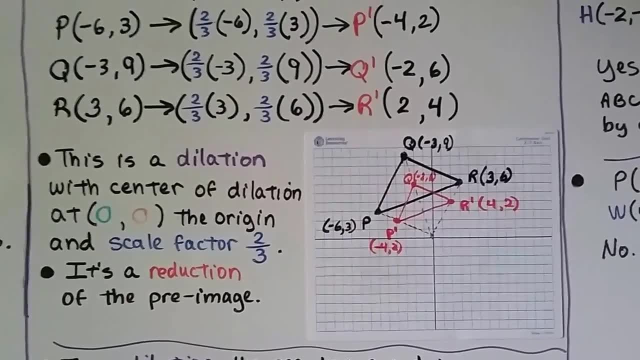 we see that the vertices go through those rays, don't they? So this is a dilation, with the center of dilation at 0,, 0 and the origin- that's the origin, and our scale factor is 2 thirds. okay, That's the value of k. 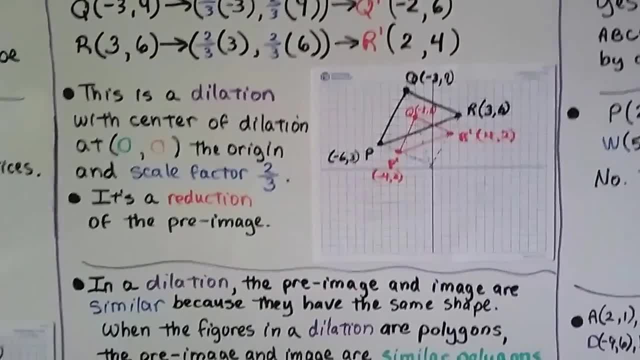 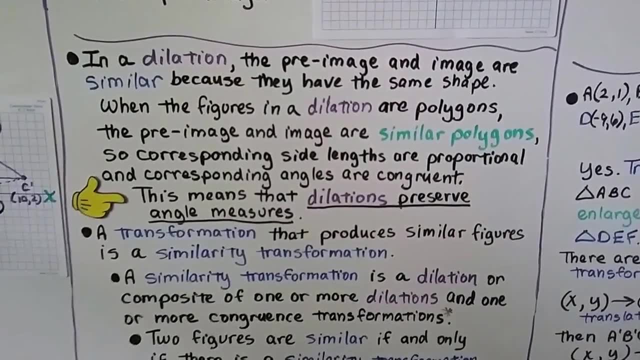 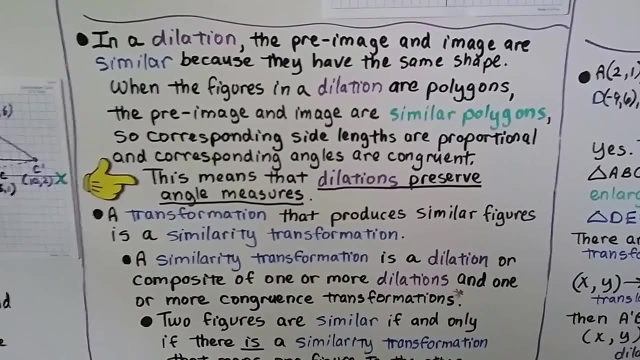 It's a reduction of the preimage. In a dilation, the preimage and image are similar because they have the same shape. When the figures in a dilation are polygons, the preimage and image are similar polygons, So corresponding side lengths are proportional and corresponding angles are congruent. 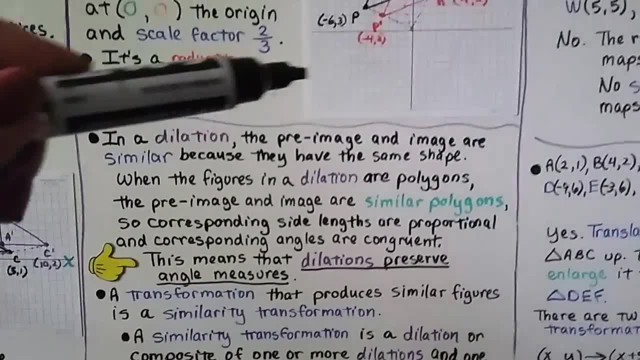 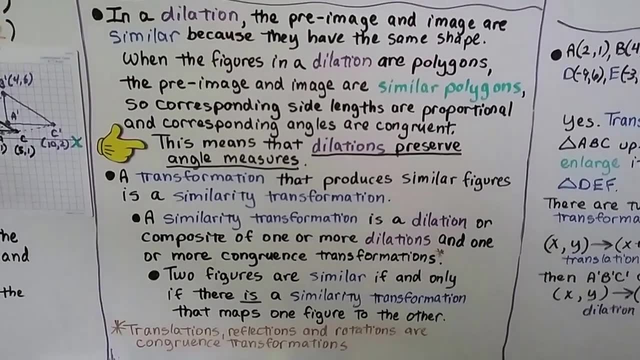 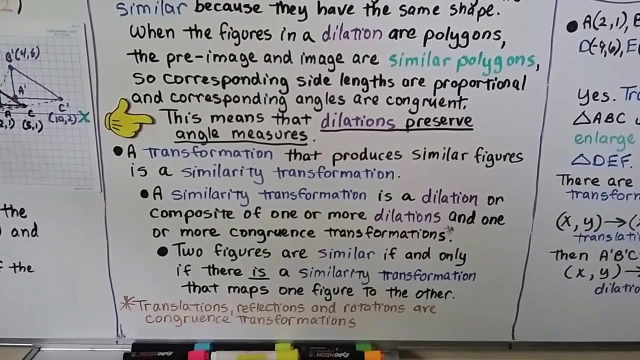 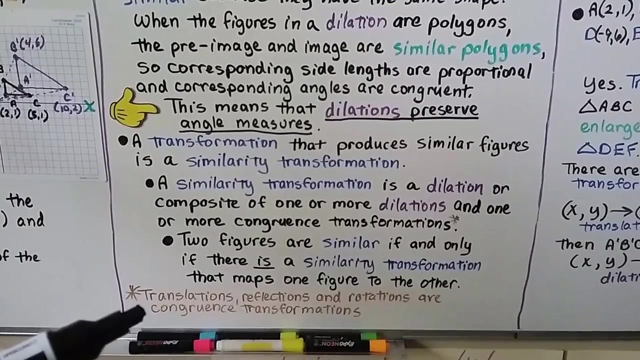 This means that dilations preserve angle measures, So the angle measure of p is the same as the angle measure for p, prime see. And a transformation that produces similar figures is a similarity transformation. A similarity transformation is a dilation or composite. It's a composite of one or more dilations and one or more congruent transformations. 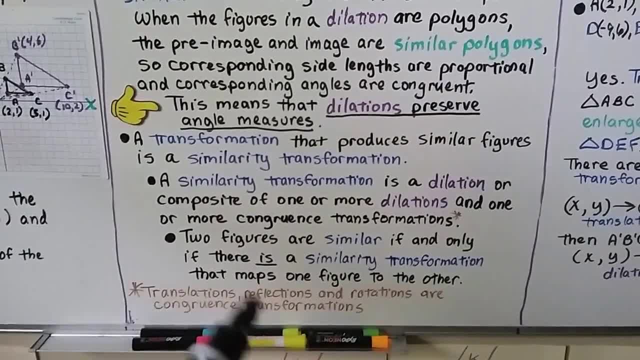 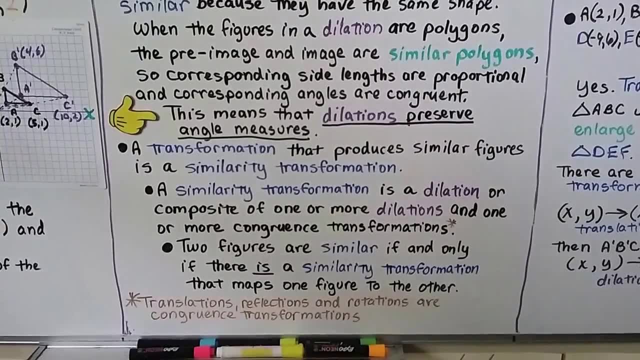 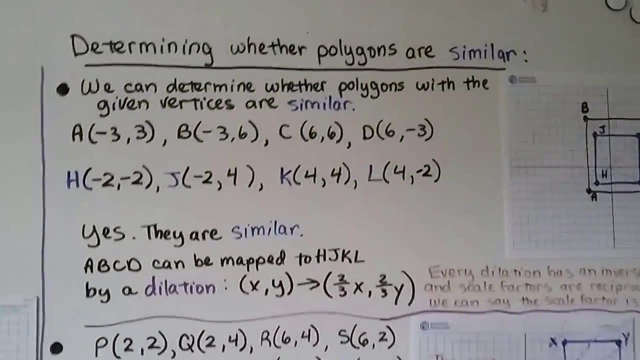 Do you remember those? Those are translations, reflections, rotations, Those are slides, flips and turns. okay, And two figures are similar? if, and only if, there is a similarity transformation that maps one figure to the other. Here's determining whether polygons are similar. 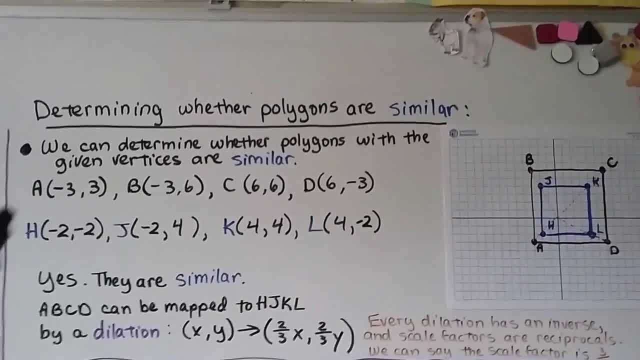 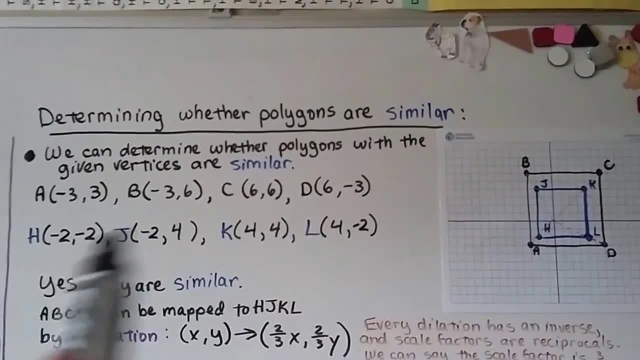 We can determine whether polygons with the given vertices are similar- A, B, C, D and the ordered pairs- and we can graph that And we got H, J, K, L, the ordered pairs. we graph that and we end up with these two triangles. 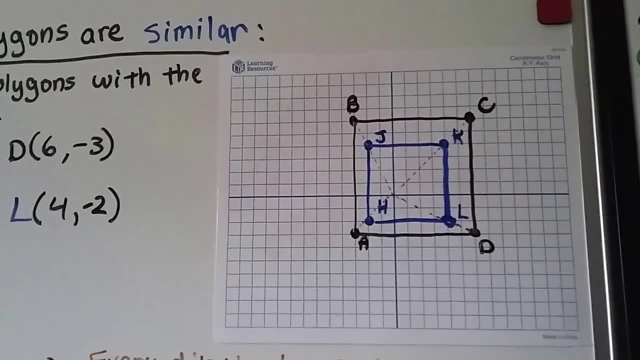 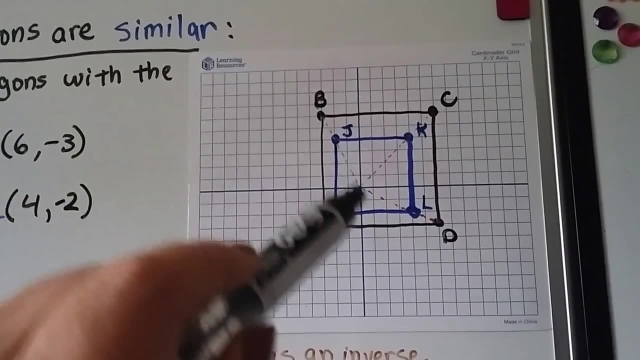 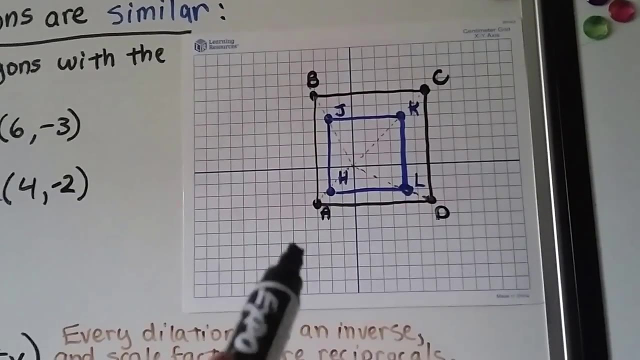 A, B, C, D is the black one and H, J, K, L is the smaller blue one, And when we draw rays from the origin through J to B, they go through the same ray and we have K and C going through the same ray and L and D going through the same one. 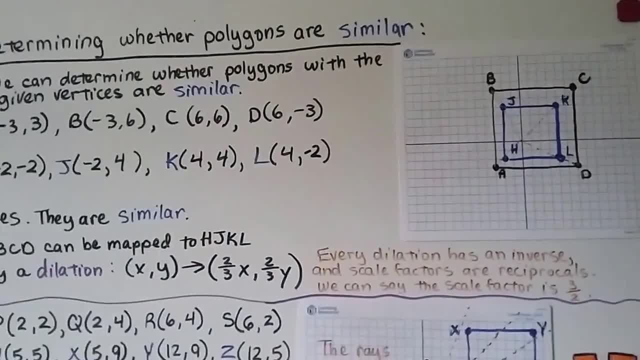 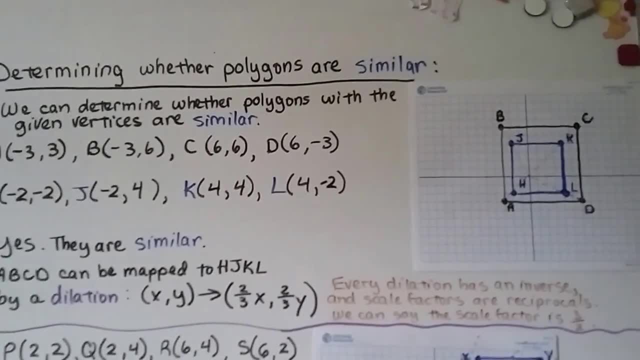 and H and A going through the same one. so yes, they're similar. A, B, C, D can be mapped to H, J, K, L by a dilation where the scale factor is a two-thirds And every dilation has an inverse and scale factors are reciprocal. 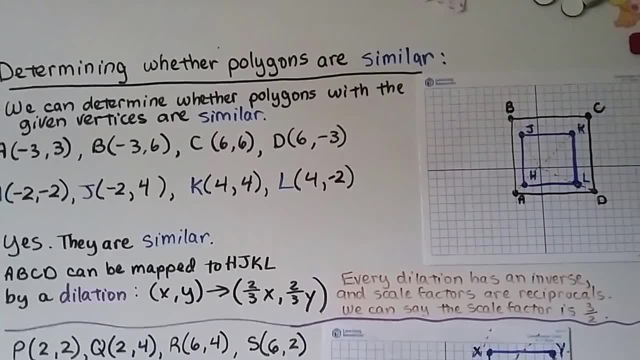 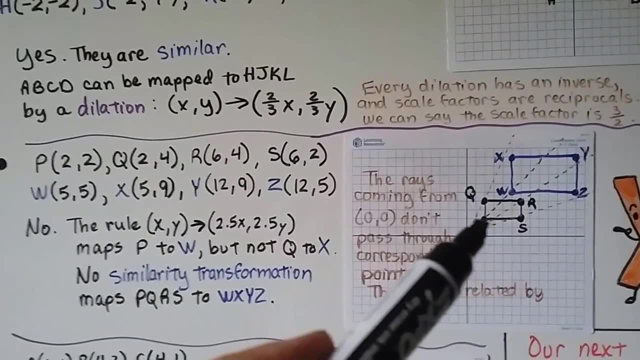 so we can even say the scale factor is three-halves. okay, Now let's take a look at this. We have P, Q, R, S, and we can plot the ordered pairs. and we have W, X, Y, Z and we can plot the ordered pairs.